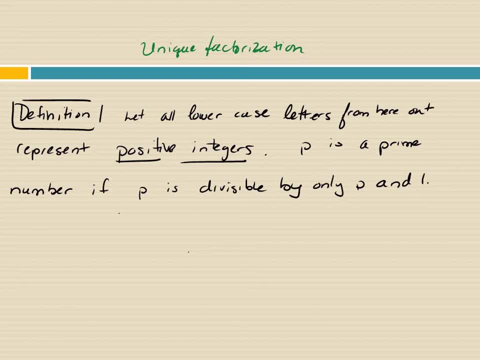 So this is what this section is about. It's one of the most important concepts in math, actually, And when I've watched students, you know one of the things that you see: students all the way up- you think: gosh. I wish I could have started over. 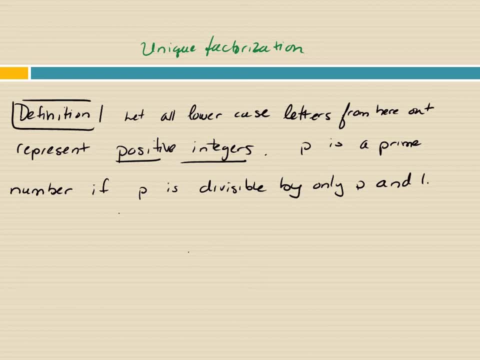 And shown them how to break things up with prime numbers and how that is important when you're combining fractions and how that relates to when you're doing algebraic fractions and how you build up in this way. And I finally got to do that experiment. I had children. 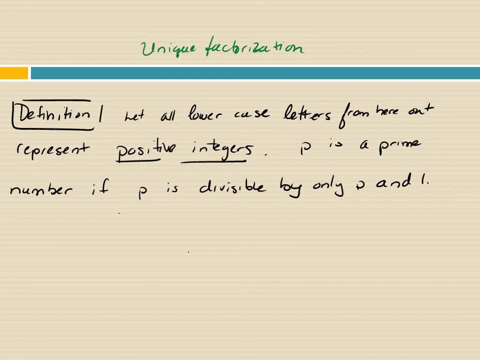 So I show my children when they're very small how to break up things into the primes, And when it comes time to add fractions, life becomes easy. Breaking up under a radical life is very easy for them because it's the same concept coming back. It is the breakdown. 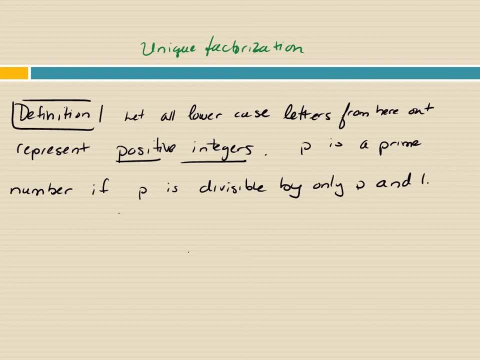 of the entire set of integers, And that's why the name of this theorem that we're going to talk about today is called the Fundamental Theorem of Arithmetic. So you're taking a step back now: Fundamental Theorem of Calculus, And now you're going back and seeing Fundamental. 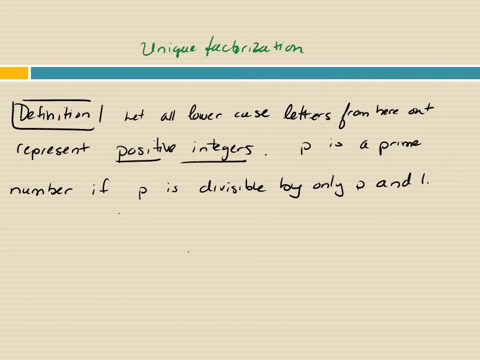 Theorem of Arithmetic. All right, so you have in this book. now he absolves himself by saying that whenever I write a lowercase letter, it's always going to mean positive integers. So he writes that at the beginning of this section. P is a prime if it is a. 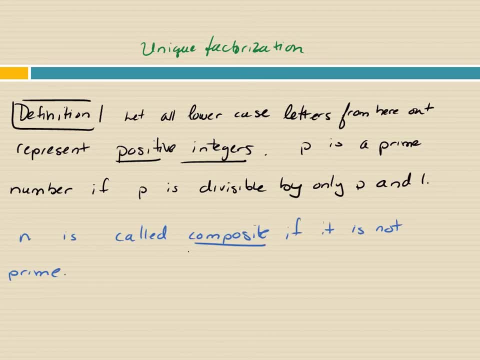 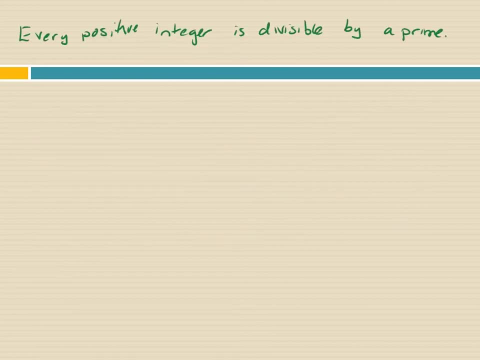 a number that's only divisible by itself, and one N is called composite if it's not prime. So every positive integer is divisible by a prime. Here's the rephrase. The top is: every positive integer is divisible by a prime. You can always state that as an if-then statement. 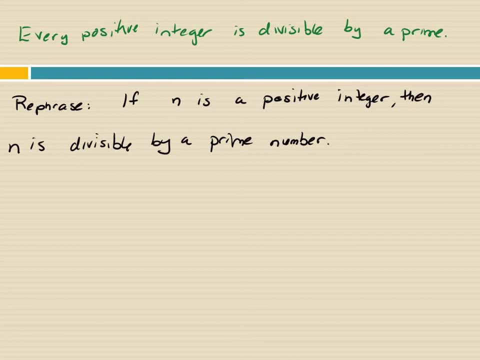 So whenever they say every positive integer, you can say: let n be a positive integer, So let u be a positive integer. If n is a positive integer, then n is divisible by a prime number. That's how you can convert it to an if-then statement. So I'm going to do this proof because 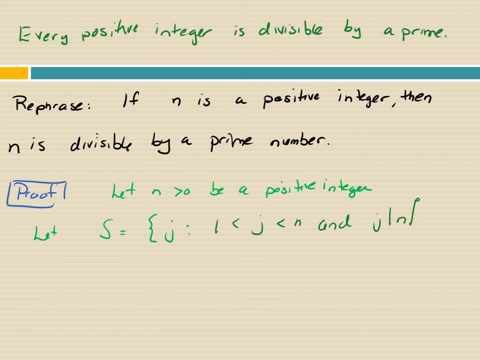 it's a concept that you see again in all your proof writing classes. If you have N as a positive integer and you want to show that it's divisible by a prime number, one of the things you can do is create a set which contains all of its divisors, And the idea is to show: 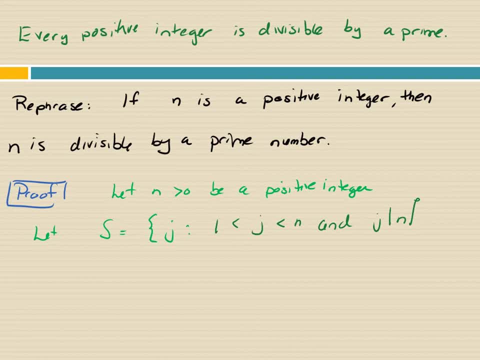 that one of the elements from that set is going to be prime, So I'm going to let s be the set of integers j between 1 and n, so it's not 1 and it's not n itself. and I'm going to show that j is divisible by. I'm going to show that one. 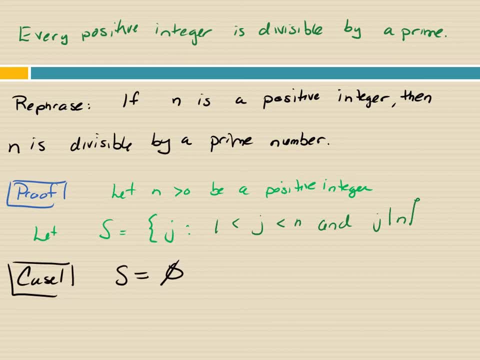 of these numbers in here is going to be prime. Well, I have two cases. One case is that there's nothing in there. Well, if there's nothing in that set, what does that mean about the number n? It's prime. It has no other divisors than itself and 1.. 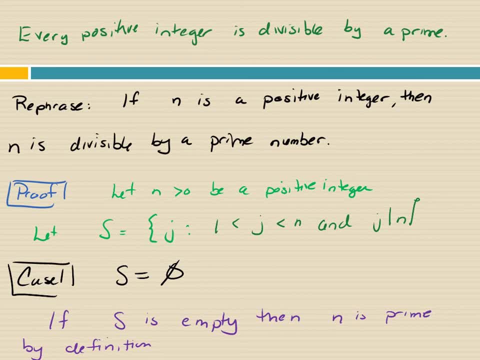 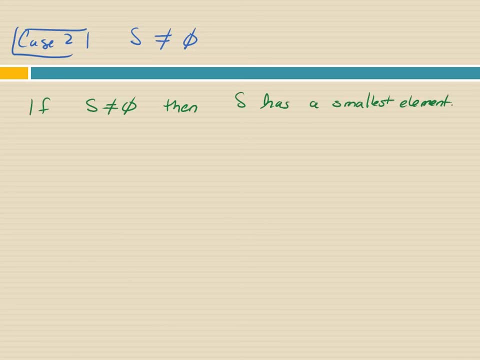 If s is empty, then n is prime by definition. What if it's not empty? Well, if s is not empty, then s has to have a smallest element. This is called the well-ordering principle, which I don't think he's talked about in here. 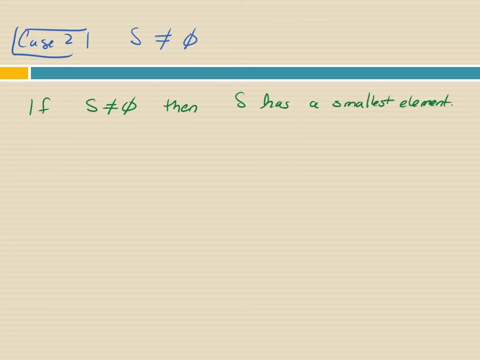 but you talk about this in a set theory class and sometimes at the beginning of modern algebra they talk about the well-ordering principle. So every finite set must have a smallest element. So I'm going to let p- I'm leading my reader here- that's going to be my candidate for. 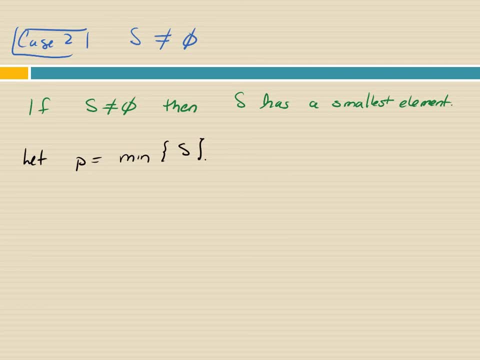 the prime be the minimum number in this set s? I claim that p is prime, Suppose on the contrary. so I'm going to do a contradiction proof. it's either prime or not. there's only two choices. Suppose on the contrary that p did have a divisor. 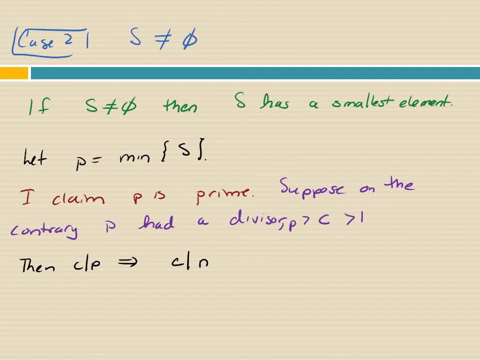 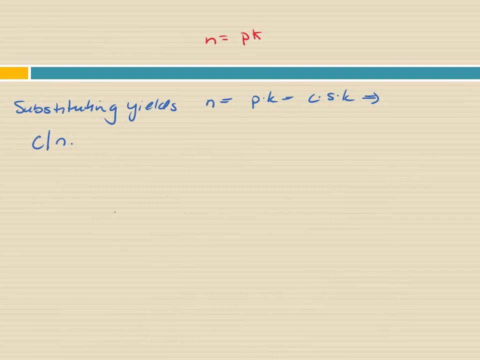 Let c be that divisor, Then c divides n as well. How do I know that? Well, I can just write down the equations and show it that if c divides p, then c has to divide n. But that's a problem because c has got to be smaller than n. 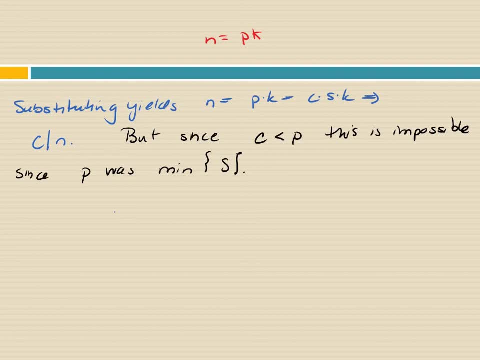 C has got to be smaller than n, because it's not prime, it's some other number that's smaller than p and bigger than 1.. So that's impossible, Because p was already the minimum, the smallest thing I could have chosen from that set s.